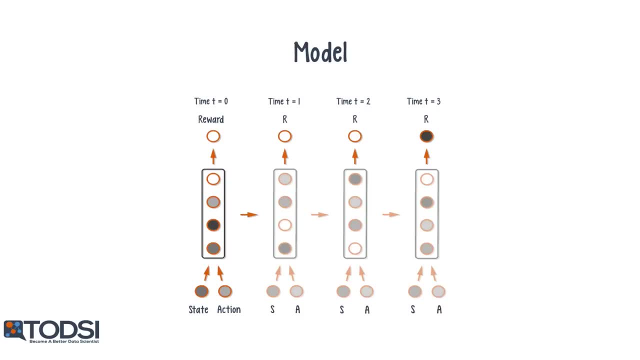 But since that only gets you to the next state, you'll need to take into account the total expected reward for every action from the current till the end state. The way this works will be different for every application, and you're probably not surprised to know that building a tennis agent. 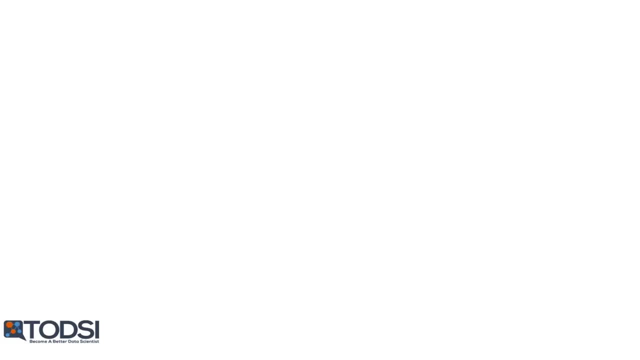 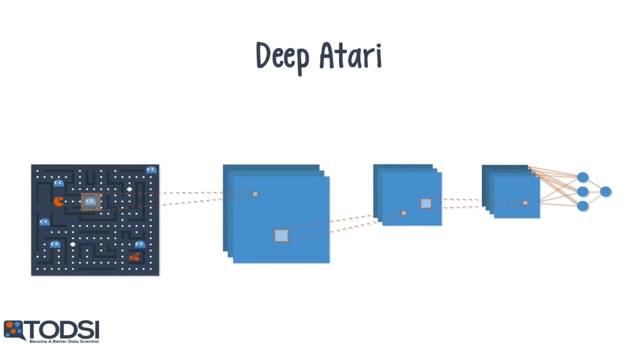 is different from building an Atari game. The researchers at DeepMind used a series of Atari screenshots to build a convolutional neural network. with a couple of tweaks, The output wasn't a class, but instead it was a target number for the maximum reward. 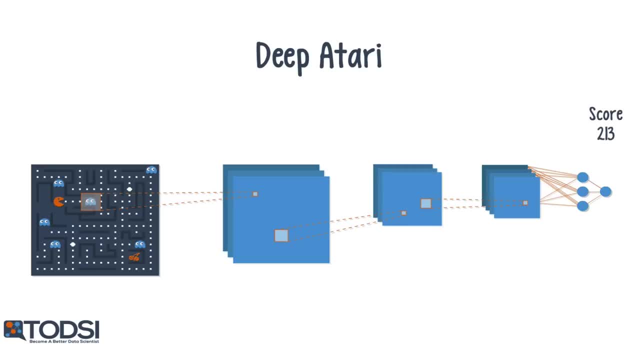 So it was actually dealing with regression, not classification. They also didn't use polling layers since, unlike image recognition, individual positions of game objects like the player are all important and can't be reduced. A recurrent net could have been used too, as long as the output layer was tailored for regression. 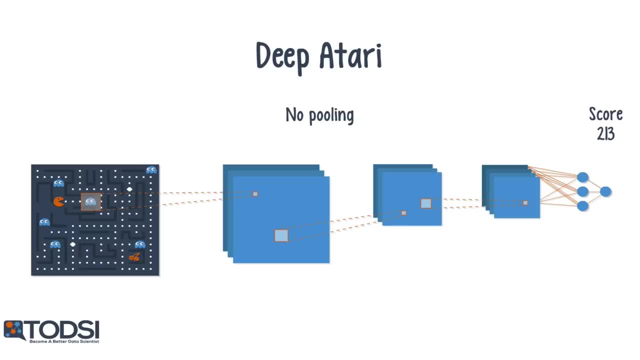 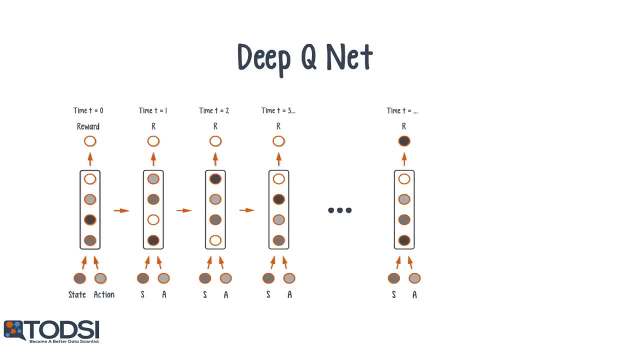 and the input at each time step included the action and the environment state. There's also the Deep Q Network, or DQN for short. The DQN also uses the principles of predicting the maximum reward given a state and action. It was actually patented by Google and it's seen a lot of improvements, like the experience replay. 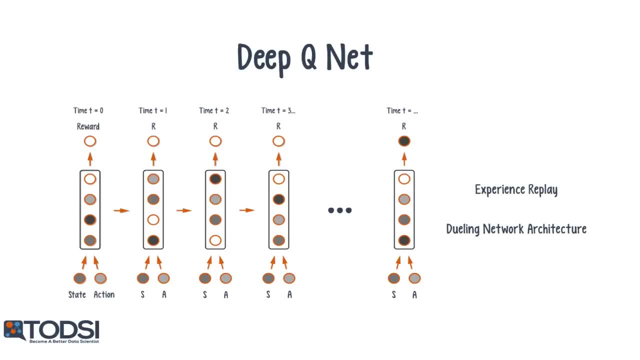 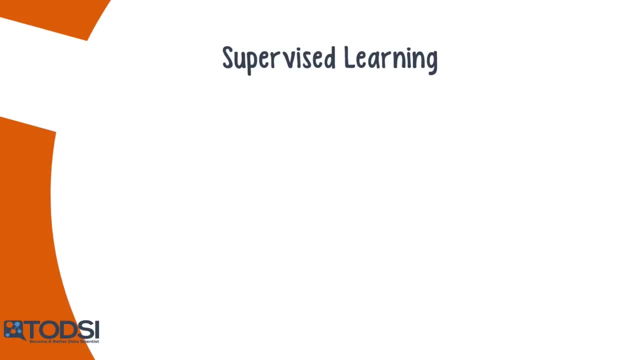 and the dueling network architecture. Reinforcement learning isn't just a fancy, smart-sounding way to say supervised learning. Supervised learning is all about making sense of the environment based on historical examples, But that isn't always the best way to do things. 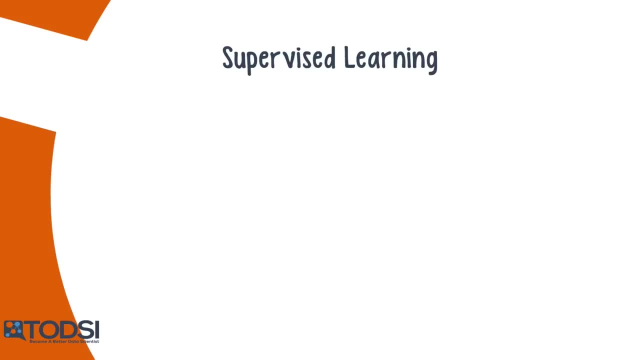 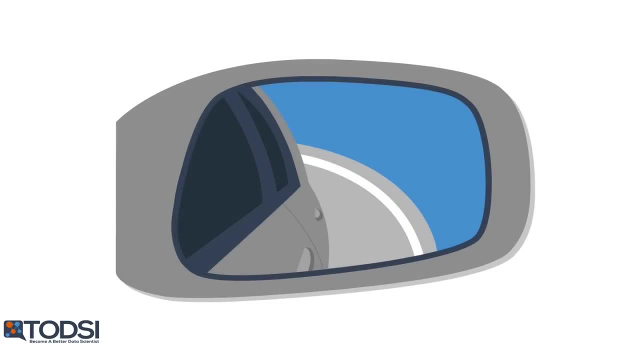 Imagine if you're trying to drive a car in heavy traffic based on the road patterns you observed the week before when the roads were clear. That's about as effective as driving when you're only looking at the rearview mirror. Reinforcement learning, on the other hand, is all about reward. 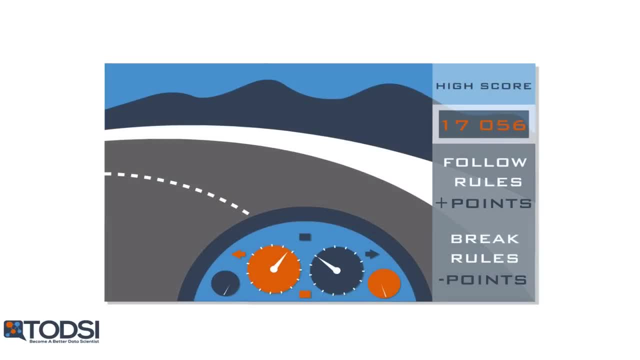 You get points for your actions like staying in your lane, driving under the speed limit, signaling when you're supposed to, things like that, But you can also lose points for dangerous actions like tailgating and speeding. Your objective is to get the maximum number of points possible, given the current state of the traffic on the road around you.